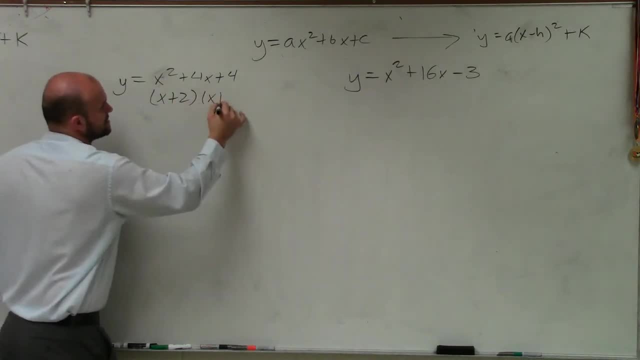 If you were to factor that into x plus 2 times x plus 2, which is x plus 2 squared, You guys see how that Perfect square trinomial binomial squared. Another example: y equals x squared plus 6x plus 9.. 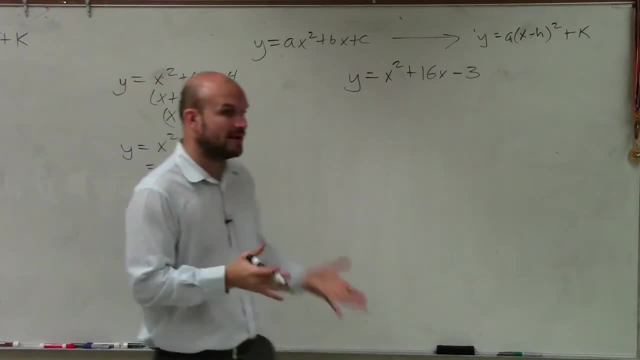 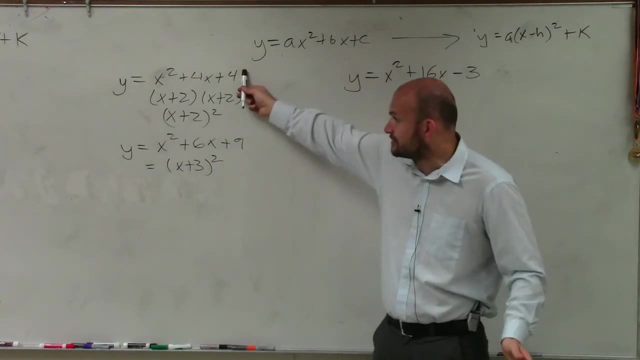 That factors down into x plus 3. That's a perfect square trinomial. So what I want you guys to understand is if we can create a perfect square trinomial, if we can create one of these perfect square trinomials. 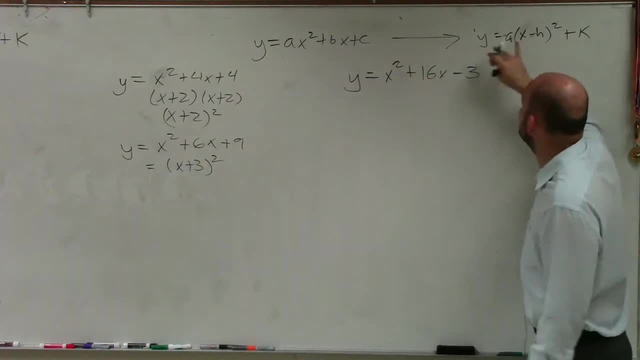 we can factor it to a binomial squared, And that's exactly what we want is a binomial squared. So we look at this: Is this a perfect square? trinomial, No, So we need to create one, And that is what completing the square is: creating a perfect. 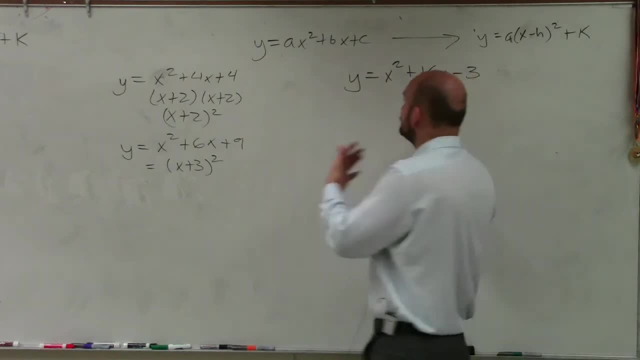 square trinomial that we can factor. So we're going to do that, All right. So how to create that? first step: make sure your coefficient is 1.. That's good for us. The next step: let's create the binomial squared. 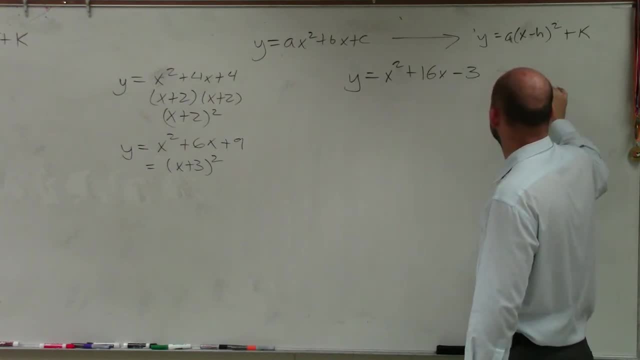 or the trinomial, perfect, square trinomial. To do that, I take b divided by 2, and I square it. In this case, my b is 16 divided by 2 squared. So therefore I have y equals x squared plus 16x. 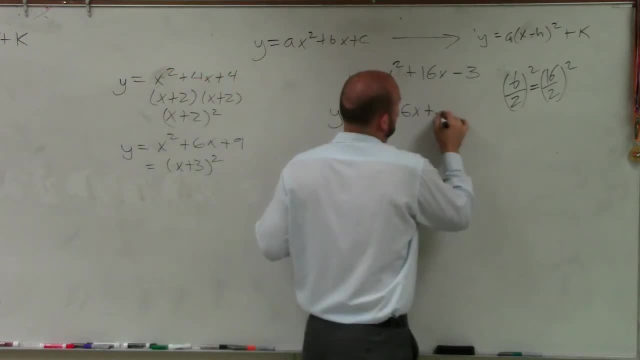 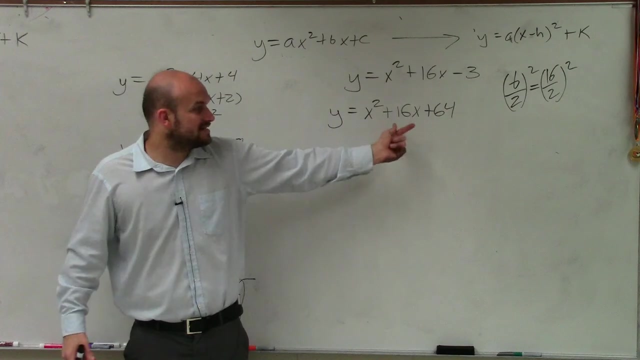 16 divided by 2 is 8.. 8 squared is 64.. 64 to the left is 64.. Do I know 1 plus 9?? Is this a binomial squared? Can I factor that out to a perfect square trinomial? 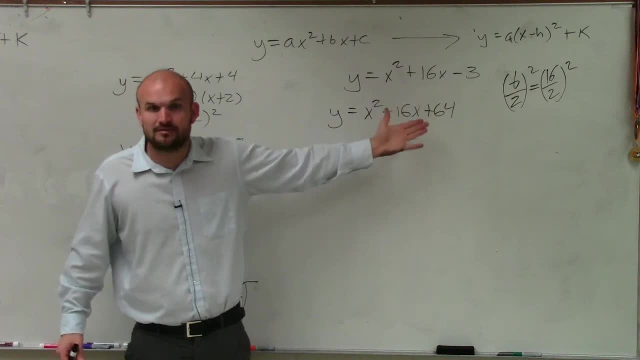 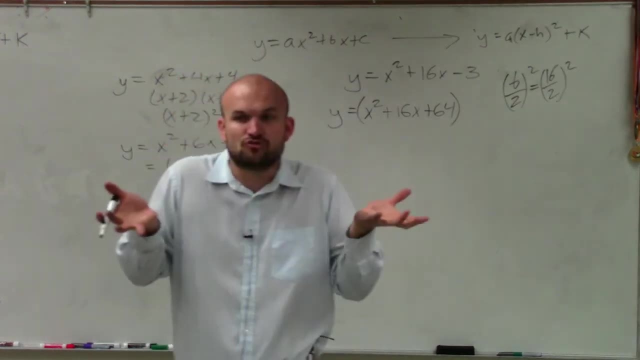 Can I factor that out to a binomial squared? Yes, I can be factored to x plus 8 squared right: x plus 8 times x plus 8? So what I'm going to do, since that's now my perfect square trinomial, I'm going to group it together. 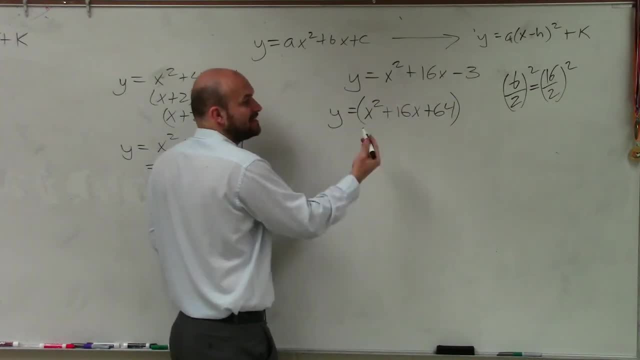 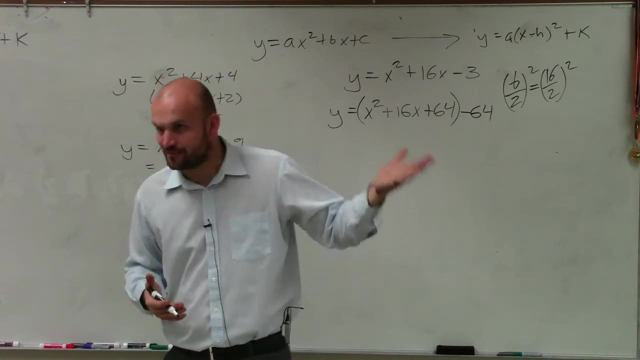 But since I have an equation and I added a 64 to one side, I have to make sure I signed 64 to the most simple assignment As heеч same side. Otherwise your equation's not going to be equal, It's going to tilt on one.